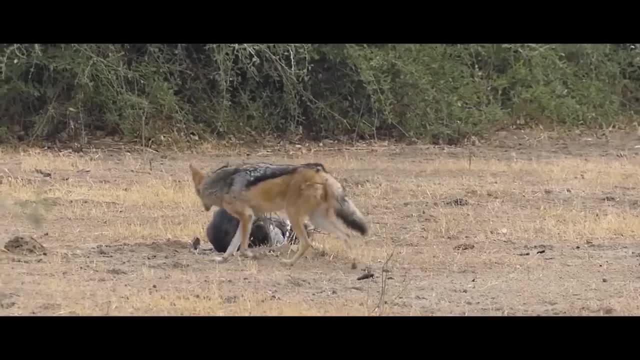 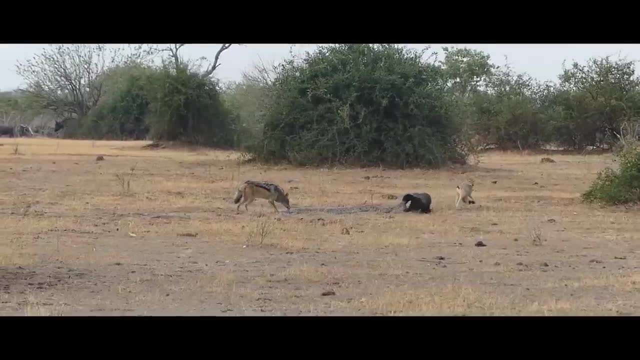 Despite the fact that only one predator ends up with the trophy, the research shows that the combined efforts of these animals increases the chances of getting food for both of them. Badgers and coyotes have the same diet and therefore they compete for food. However, the cunning prairie dogs are not easy to catch. They are not easy to catch, so the coyote can't catch the prey. However, the cunning prairie dogs aren't easy to catch. They can't catch prey if they don't get the prey. 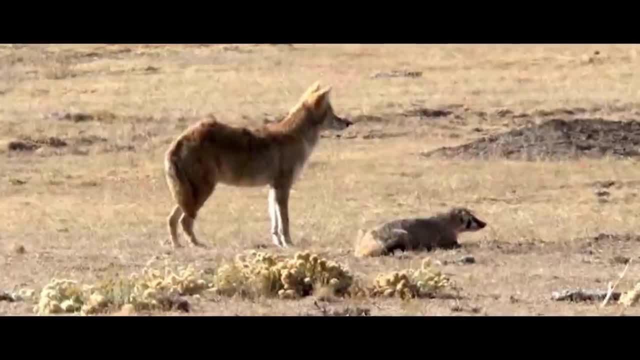 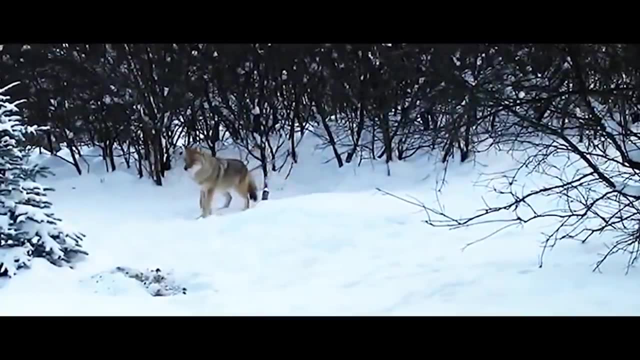 However, the cunning prairie dogs aren't easy to catch. They can catch prey if they don't to catch, as they rarely stray far from their burrows. So the mighty badger-coyote alliance actually helps both animals improve their odds when 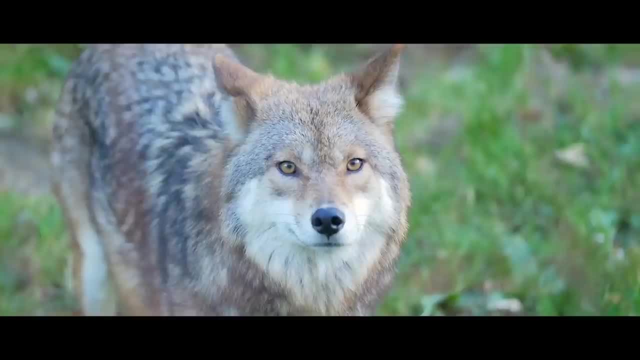 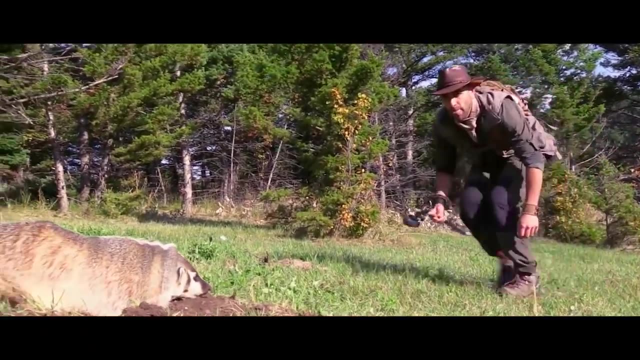 hunting the prairie dogs. Some coyotes band into free communities, but the majority of them lead a solitary lifestyle as they rarely hunt in packs. Interestingly, a badger is even more of a loner than a coyote is, which makes their 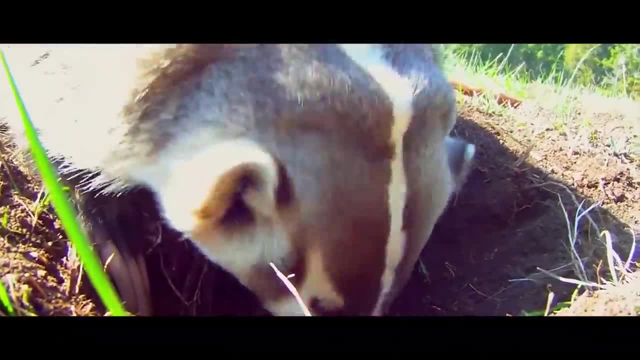 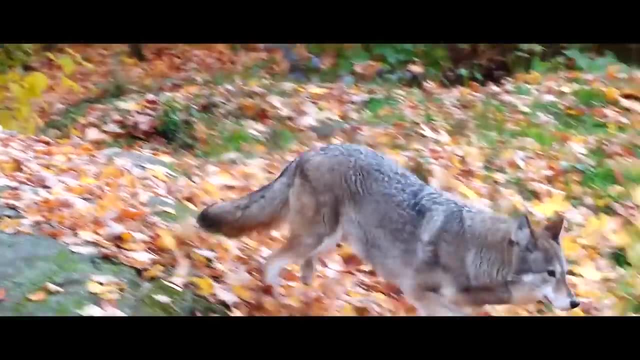 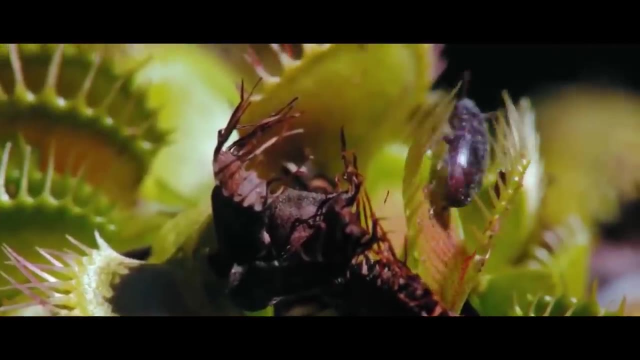 partnership even stranger. The research demonstrates that those coyotes who cooperate with badgers catch about one-third more prey than those coyotes who prefer to hunt on their own Carnivorous Plants and the Bat Feces. Carnivorous plants devour and digest living organisms that end up caught in their traps. 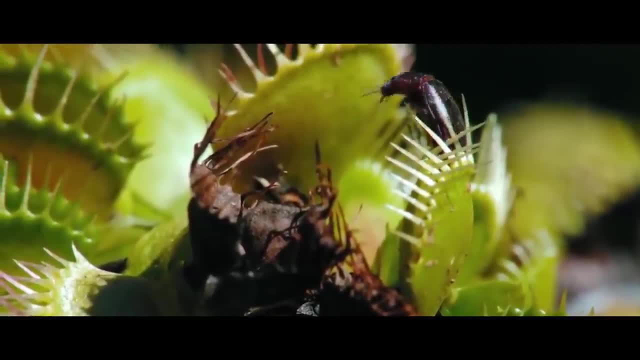 Carnivorous plants have evolved to consume this type of food owing to a lack of nitrogen. Similarly to how a Myomrocodea attracts ants to use their food to hunt, carnivorous plants have evolved to consume this type of food owing to a lack of nitrogen. 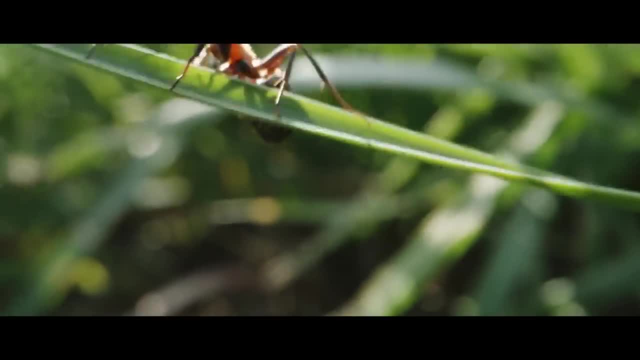 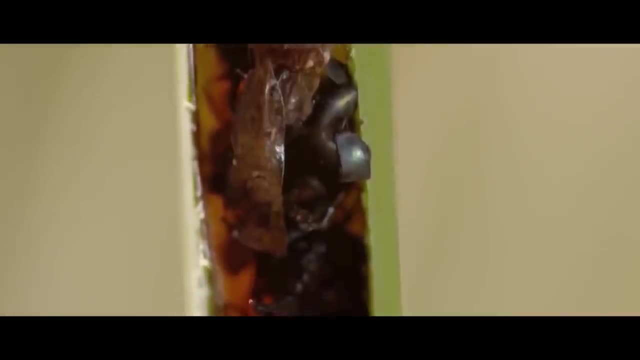 In addition to the fact that carnivorous plants eat their nitrogen-saturated waste products, the predatory carnivorous plant usually lures in insects and small animals. In this case, however, the plant doesn't offer shelter to its guests, but rather consumes them instead. 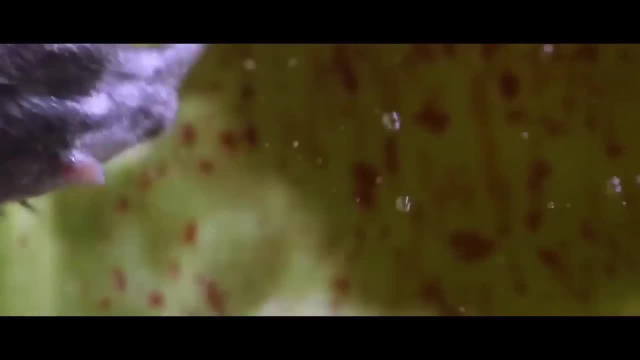 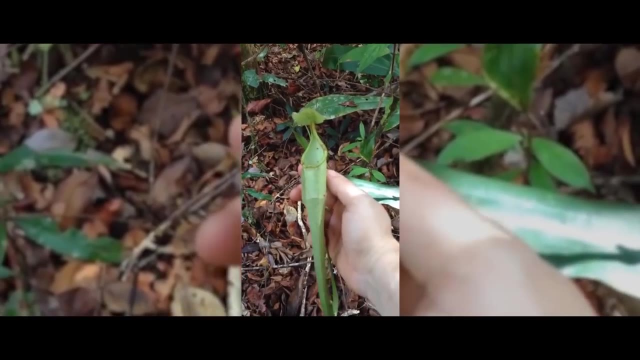 Nevertheless, there is a type of carnivorous plant species that is very hospitable. Nepenthes hemsliana is an unusually large plant of this type, which learned to coexist with bats During the day, Vespertilianae bats of the Caryoptera, which are the largest of the 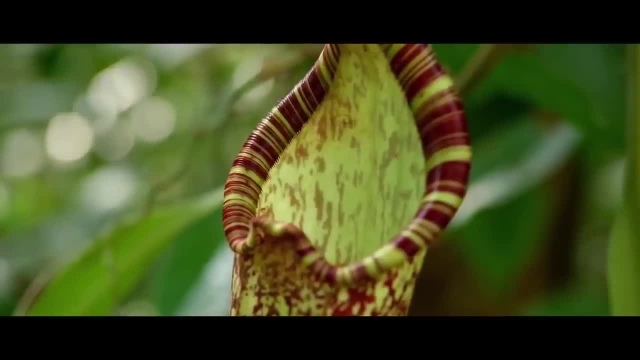 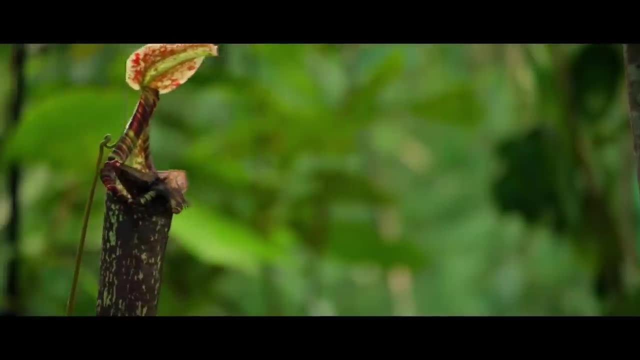 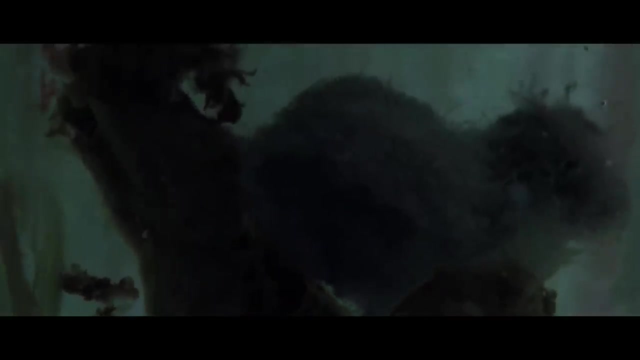 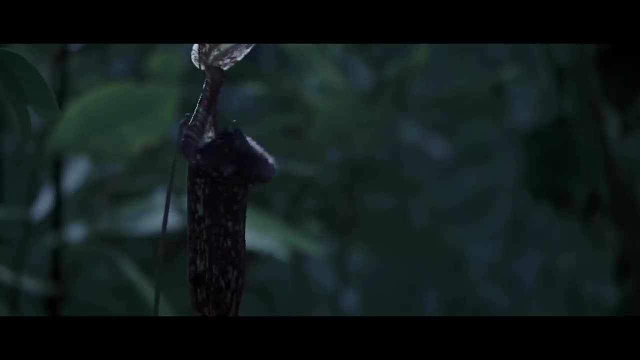 Caryvula hardwickii kind enter the plant and rest there until nightfall. Contrary to expectations, the plant doesn't digest their guests, but are actually happy to shelter the bats to recycle their feces later. There is a reason why bats choose this specific plant out of the rainforest-rich canopy. 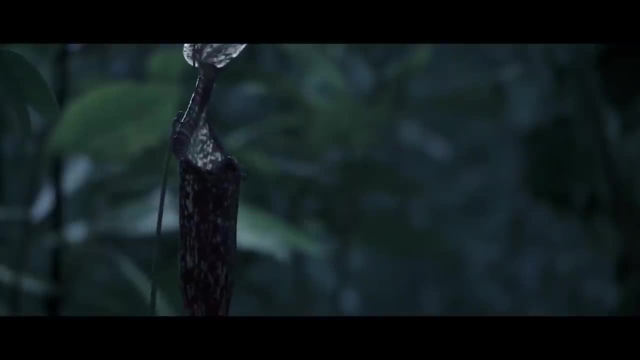 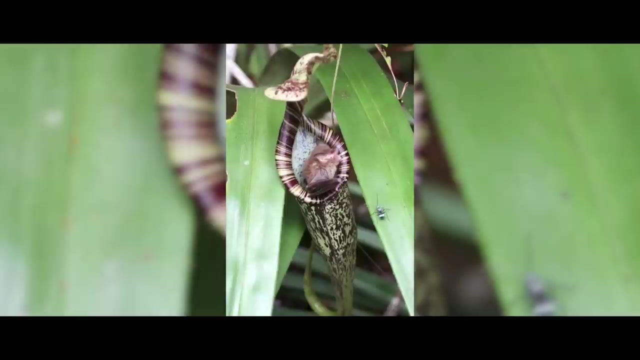 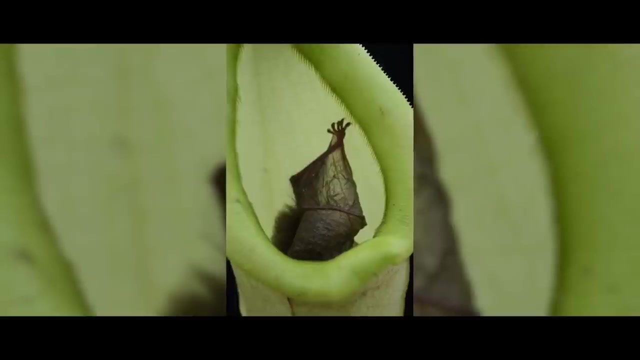 This carnivorous plant has its special ways to attract the bats. The backside of the Nepenthes flower is saucer-shaped and can reflect the signals emanating from the bat who's searching for shelter. Thus the echolocation leads the bat straight to the giant flower and both sides benefit. 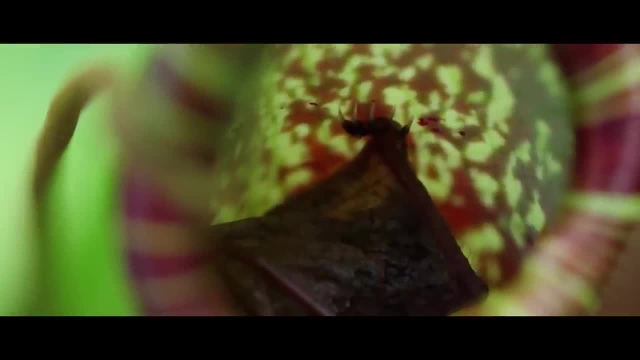 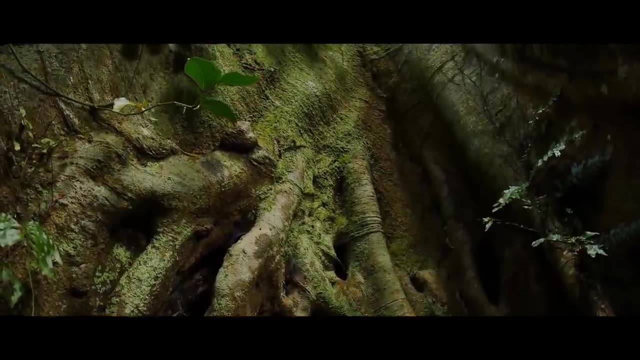 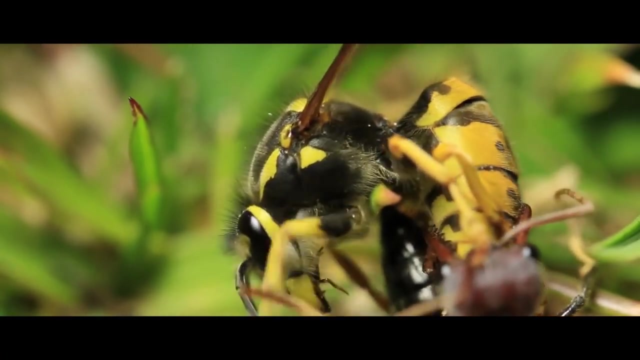 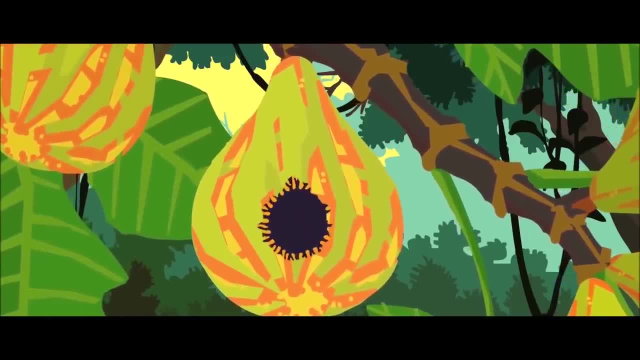 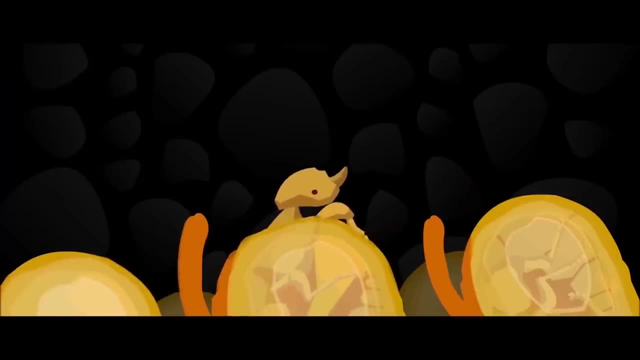 The relationship between these insects and fig trees started 60 million years ago at the very least, So it's not like the wasps get in our way of enjoying figs, but, on the contrary, we are the invaders of their comfort zone. By the way, 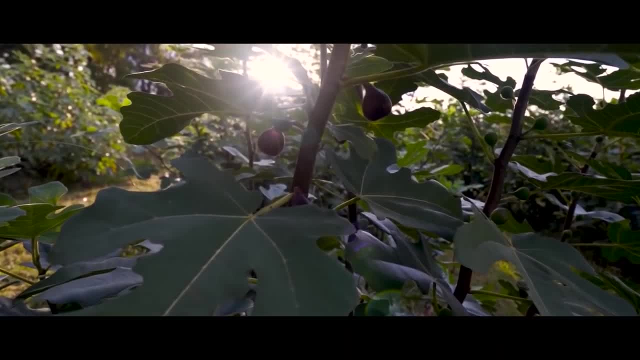 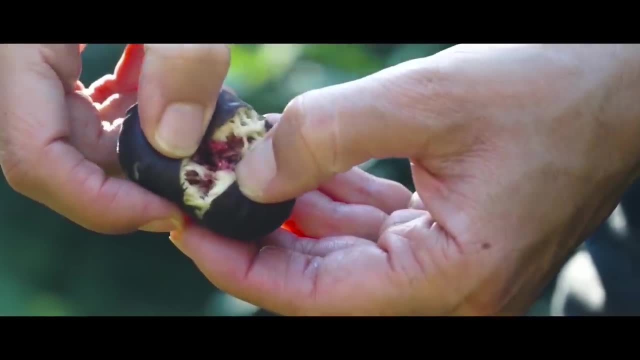 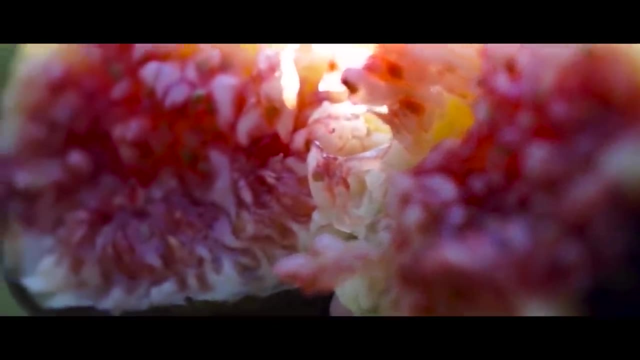 A fig is not exactly a fruit. There's no fruit: a hollow, roundish structure composed of a multitude of flowers. As the fig matures, it emits a smell that attracts the pregnant wasps from the family Chalcedoidae. The insect must literally burrow its way inside the fig. This is actually harder than it sounds, and the wasp often ends up tearing its tentacles and wings in the process. As soon as the wasp gets inside, it lays eggs there and also brings in pollen from other fig trees. Once the mission is accomplished, the wasp dies. 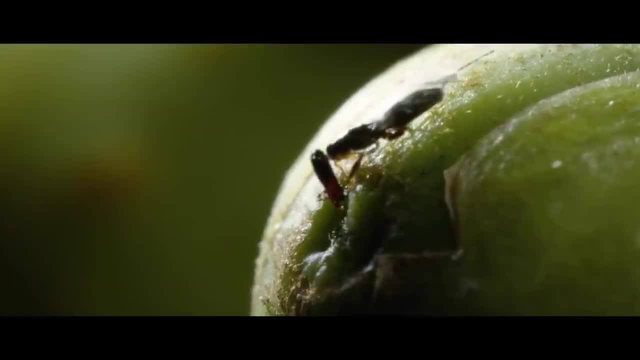 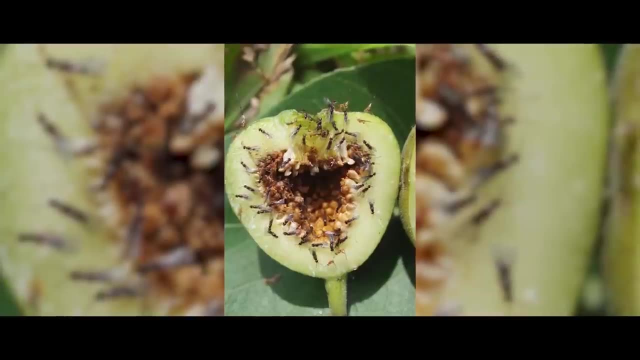 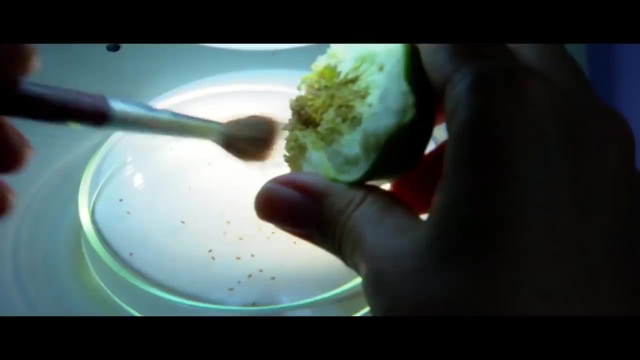 If a fig tree doesn't get pollinated, it hibernates and ultimately dies together with the wasp eggs. This is a cruel way that evolution has designed to ensure that wasps pollinate fig trees, as the lives of all wasp eggs depend on it. 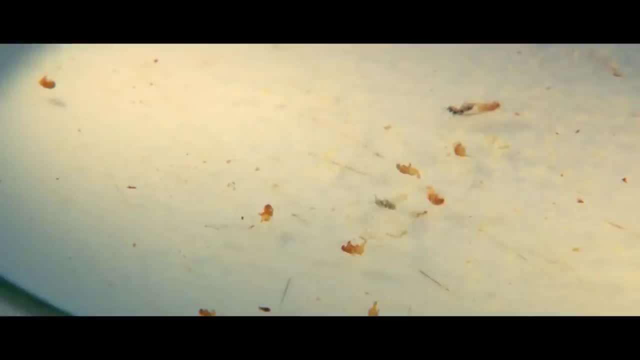 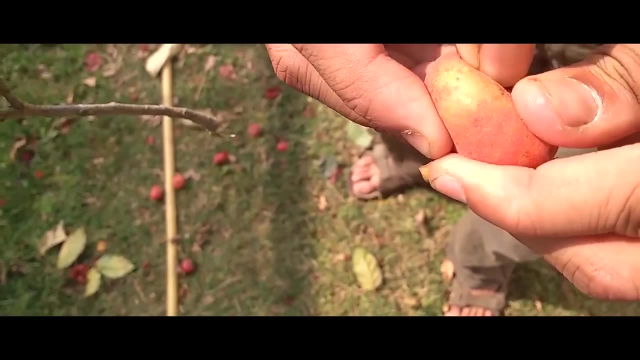 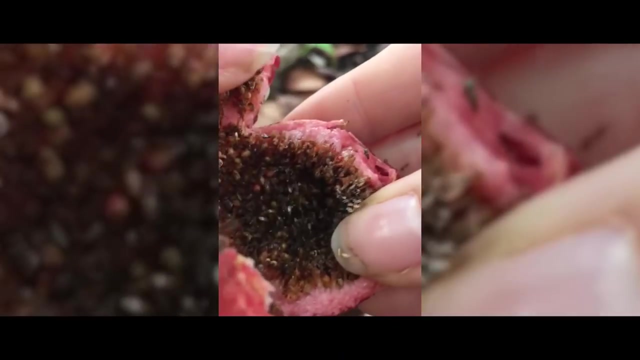 If pollination does happen, then the fig eventually splits and a new generation of wasps hatches. At first they feed on the fig pulp. Both male and female wasps grow inside the figs. Male wasps collect the pollen for female wasps and dig their way out of the fig. 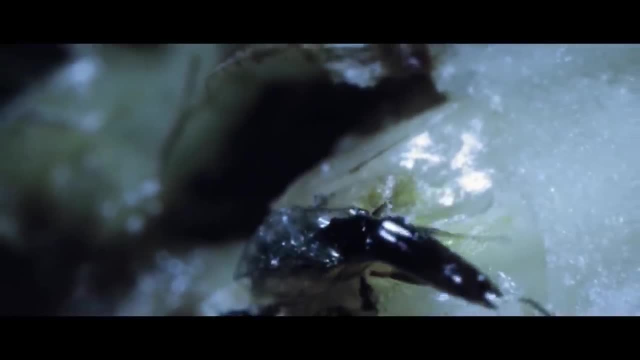 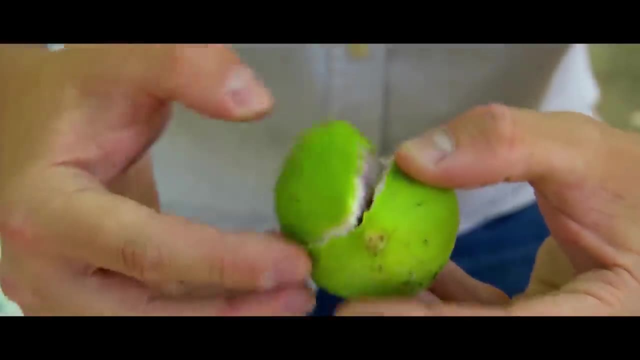 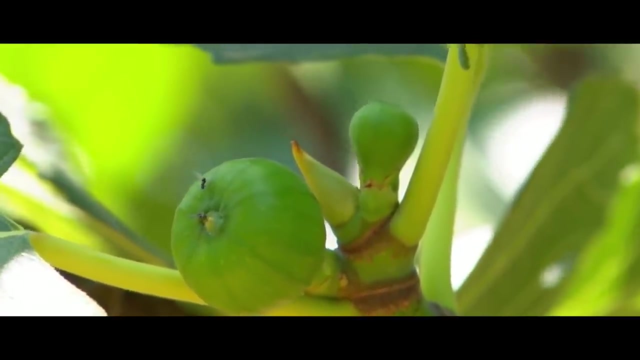 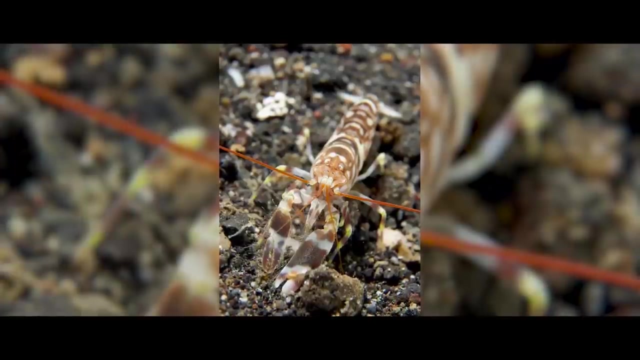 Males succeed in bringing pollen from the other plants before female wasps break free and go out in search of a new fig tree to lay their eggs in. Thanks to this cycle, both plants and insects continue to thrive. Goby Fish and Pistol Shrimp. Goby Fish and Pistol Shrimp are best pals on. 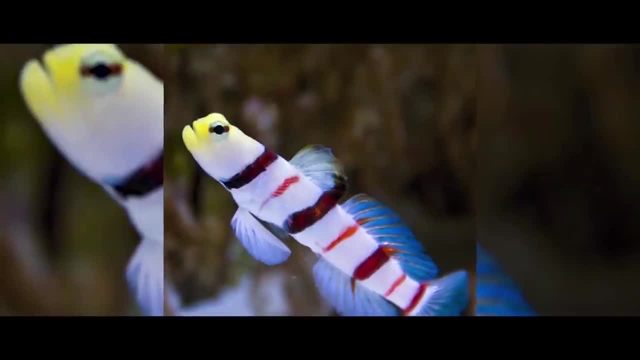 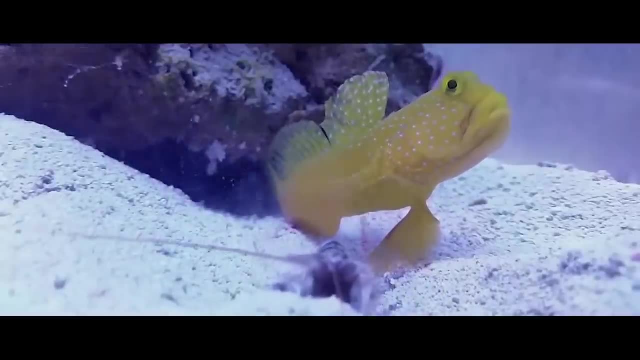 the ocean floor. Almost like roommates, these two different creatures have a clear-cut and clean symbiotic relationship. Pistol Shrimp don't object to sharing its home with Goby Fish, As the former builds a home for them on the sea floor. the latter observes the environment. 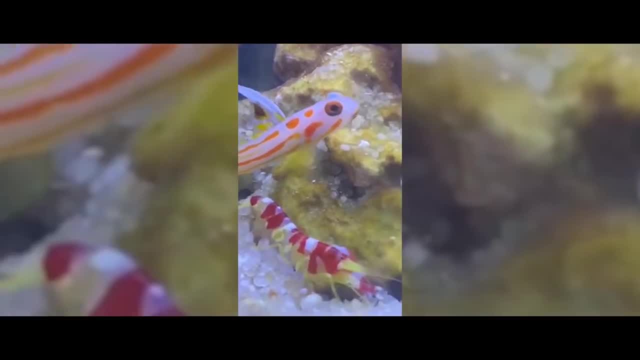 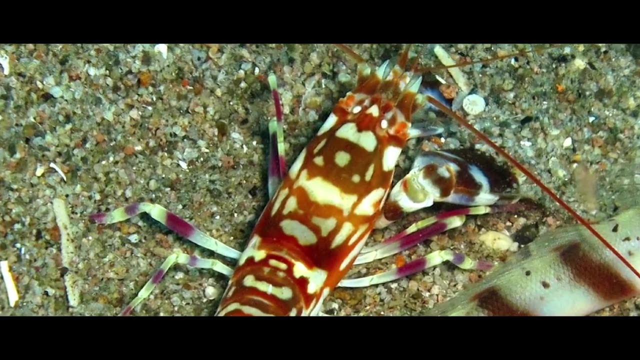 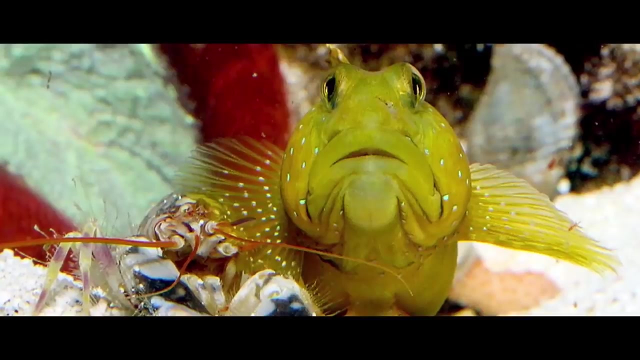 defending both the burrow and the Pistol Shrimp. The Goby Fish has excellent eyesight and can easily spot an enemy, giving an advanced warning to the Pistol Shrimp. Thus, these two creatures share a mini-cave under the sea and help each other out. 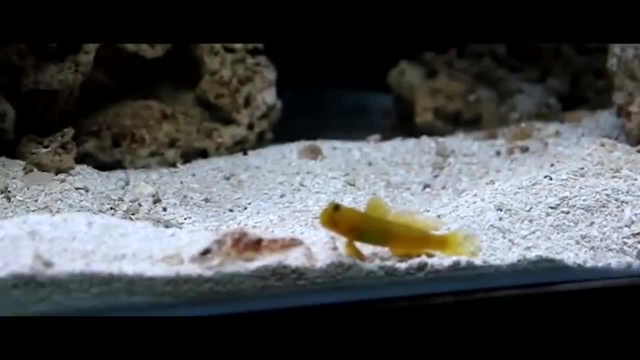 Pistol Shrimp and Pistol Shrimp, Since Pistol Shrimp and Pistol Shrimp have a very close relationship. they have a very close relationship Since Pistol Shrimp are mostly blind. they let the Goby Fish know when they are about to leave their home in search of food. 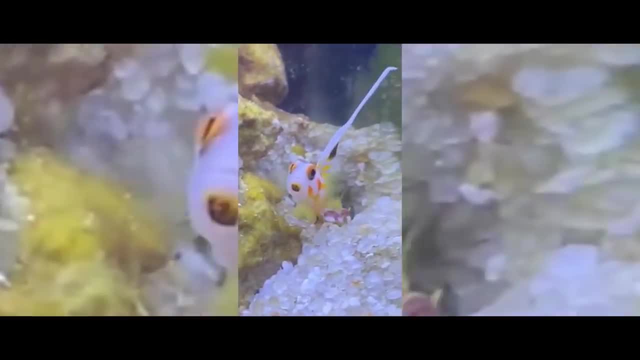 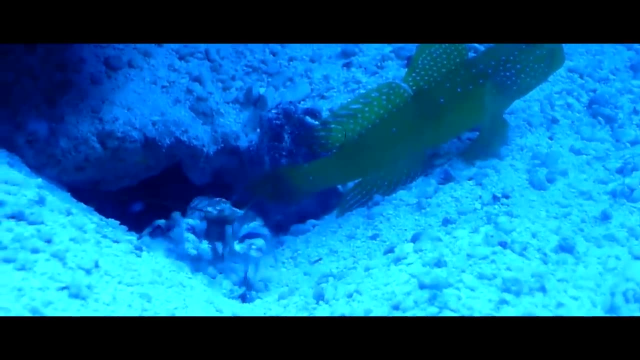 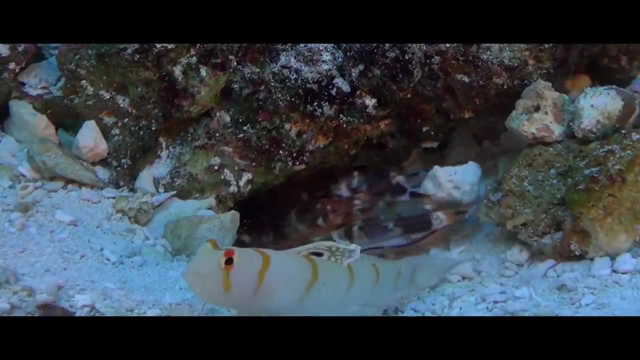 Then, as they move, the Pistol Shrimp touch the Goby Fish with their antennas, continuously maintaining contact. Pistol Shrimp populate shallow sea beds and it is important for them to maintain symbiotic relationships with the Goby Fish. It has been noted that the Goby Fish even collect seaweed and other food for their roommates. They can bring seaweed to the burrow sometimes, but they can't bring seaweed to the sea. The Goby Fish have a very close relationship with the Pistol Shrimp. The Goby Fish have a very close relationship with the Pistol Shrimp. 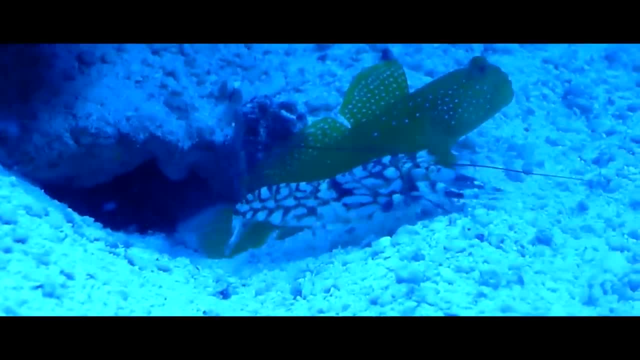 It is important for them to make sure that the Pistol Shrimp does not throw goby fish at the burrow. They must find the top of the burrow and the bottom of the burrow to get out of the net. They must bring seaweed and other food in the burrow to stay away from the Goby Fish. 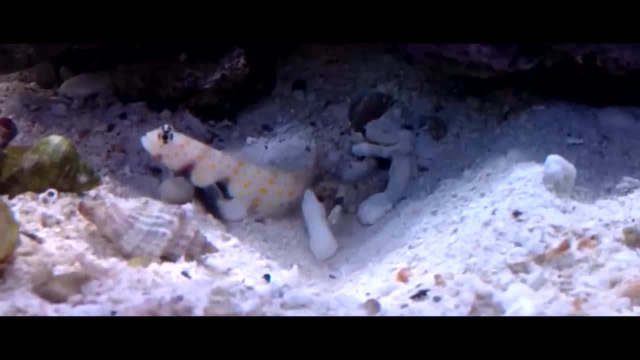 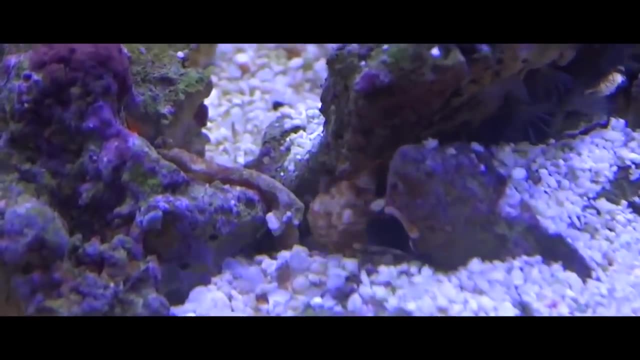 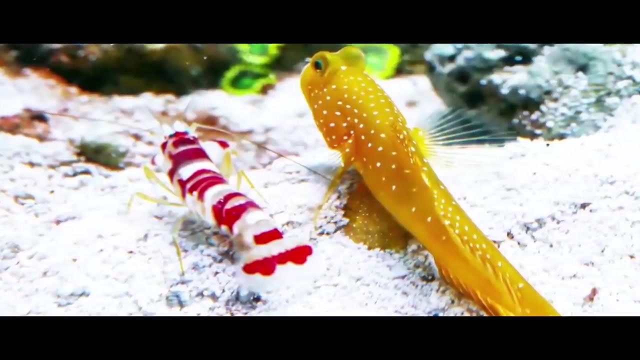 If the Goby Fish sees danger lurking around, they snap their tails as a sign of warning. In exchange for protection, the Pistol Shrimp provide their guards with shelter. The Goby Fish also use the burrow's safety to seduce its partner with a special ritual. 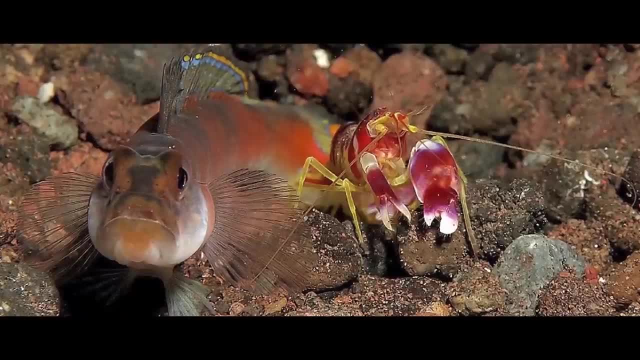 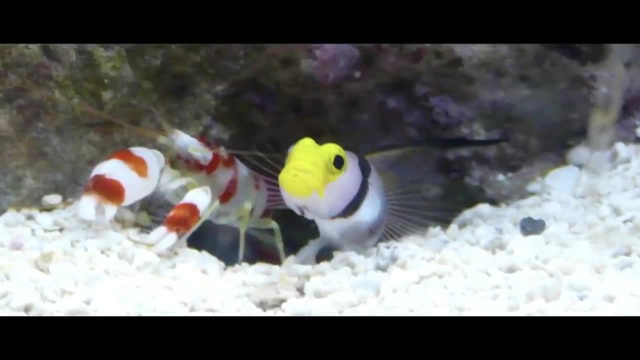 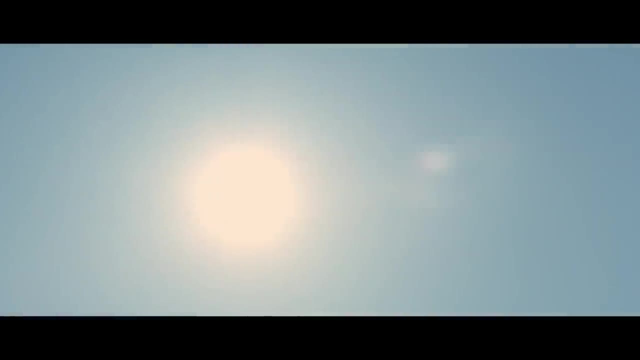 which lasts for quite some time. Astonishingly, over one hundred types of Goby Fish maintain symbiotic relationships, and their relationship is very close with pistol shrimp, The Warthog and Mongoose. Once upon a time, Ugandan scientists witnessed a strange friendship between warthogs and 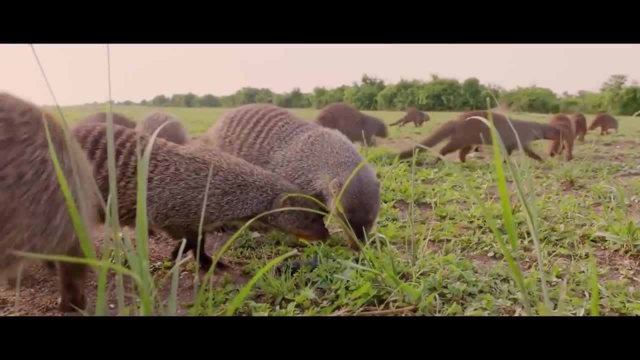 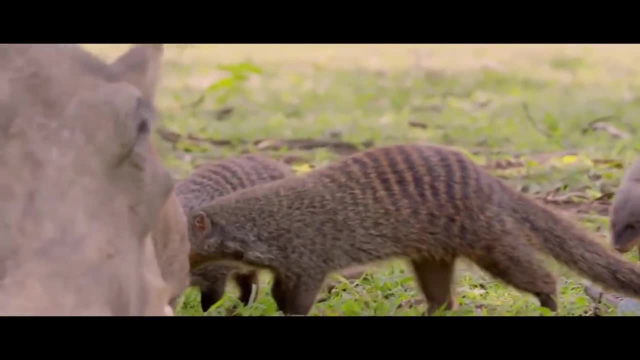 mongooses. The scientists of the Ugandan Queen Elizabeth National Park noticed that warthogs lie down on the ground once they come across a mongoose. Thus, warthogs are treated to a fastidious clean-up as sharp-toothed mongooses collect. 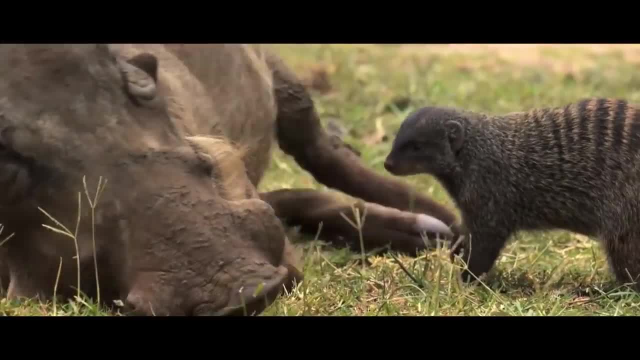 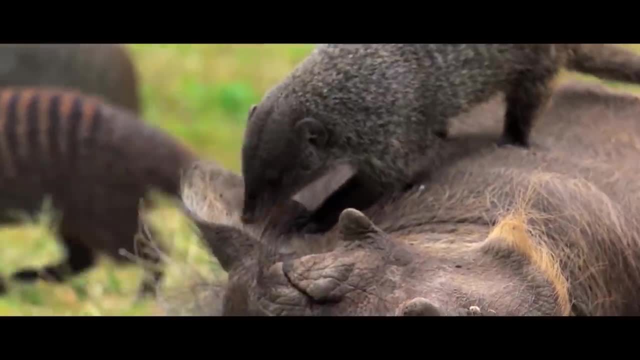 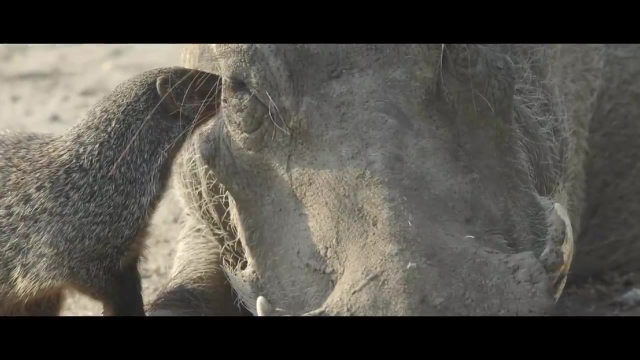 insects, and especially mites, off their skin. So a mongoose eats while a warthog gets some thorough cleaning. Often a group of mongooses clean the warthog's rough skin together with some of them even mounting the pig, The African Swine. 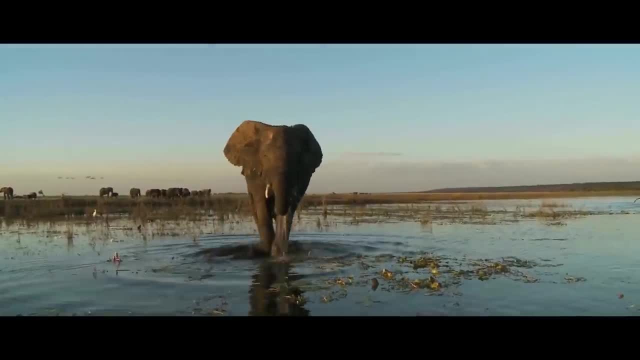 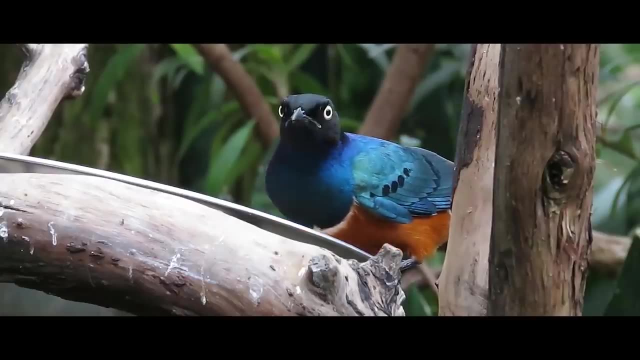 African starlings spend a great deal of their time sitting on elephants, rhinos, zebras and African buffaloes, where they eat mites picking them off their host's skin. This diet provides the African starlings with all the nutrients they need. 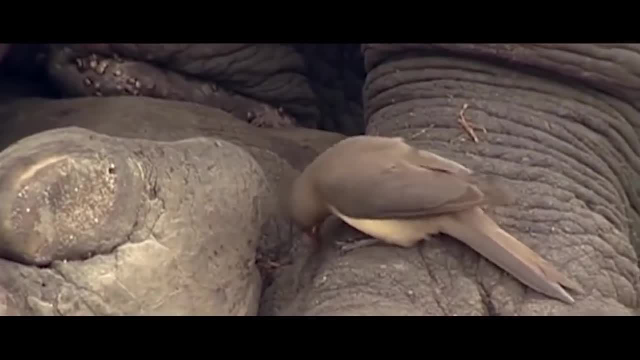 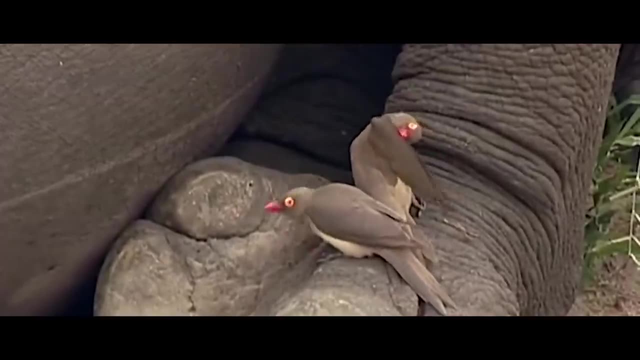 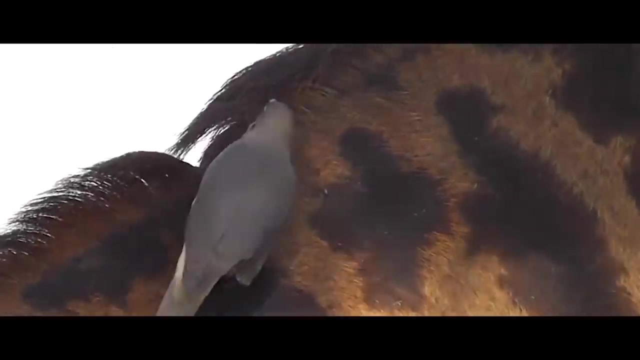 Besides, big animals are elated that the birds free them from the parasites and mites. Scientists believe that this relationship started a very long time ago, as it seems that the starlings' beak was created exactly for the purpose of deep penetration into the animal's skin. 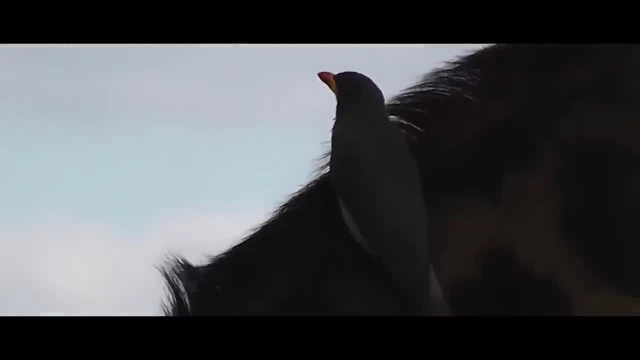 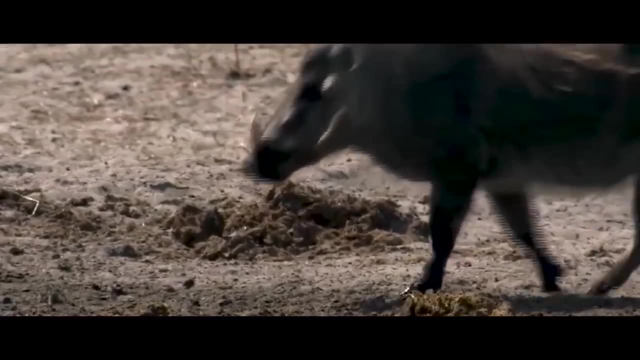 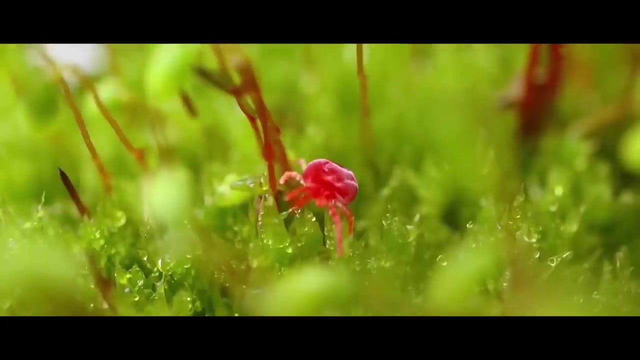 to search for food there. However, the relationship between African starlings and their host animals aren't always mutually beneficial. When starlings remove the pests from the animal's skin, they also suck some blood from the open wounds. That's another way to obtain nutrients for them, but it also makes the birds into parasites. 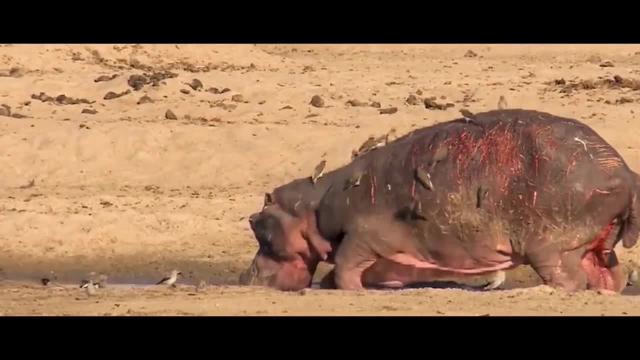 This practice might lead to an increase in the number of starlings that come into the animal's skin. This practice might lead to an increase in the number of starlings that come into the animal's skin. Later. it probably leads to infection of the host animal, blurring the symbiotic.